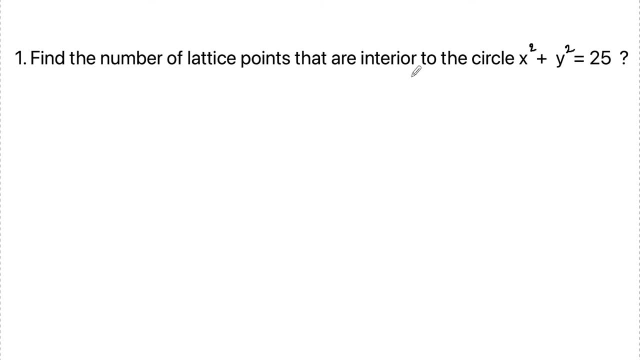 Find the number of lattice points that are interior to the circle x square plus y square is equal to 25.. So what are lattice points In x- y coordinate system? in x- y coordinate system, point x comma y is called a point lattice when x and y are integers. So given interior. 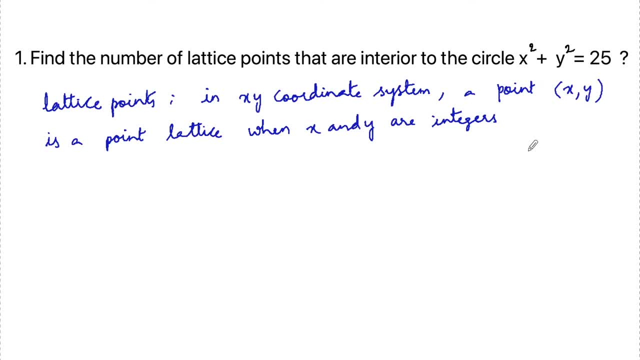 to the circle. x square plus y square is equal to 25.. So x square plus y square is equal to 25, is a standard circle with radius 5 units. x square plus y square is equal to 5 square. The radius of the circle is 5 units and its 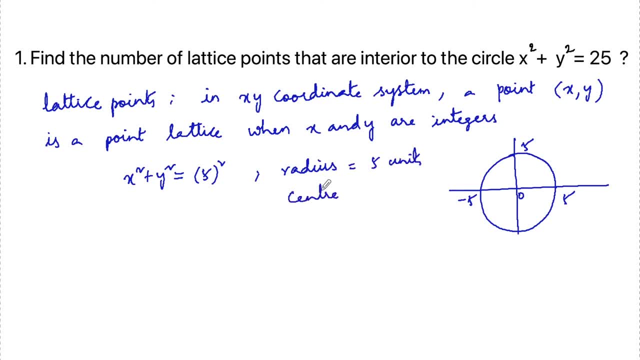 center is origin, 0 comma 0.. Center of the circle is 0 comma 0. And we need to find each and every point which is inside. and that too, lattice point Means we need to find the integral points like x comma y, such that x and y are integers. 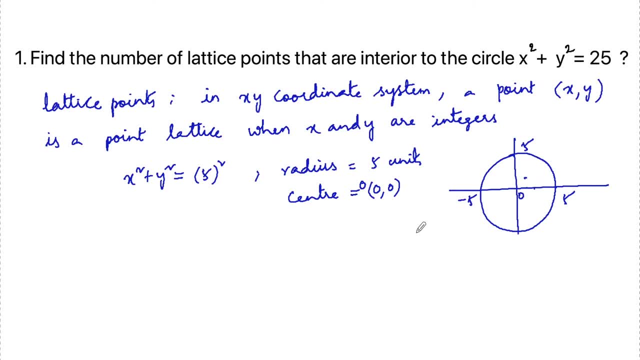 Like an example: 1 comma 1, 1 comma 3.. So which are which will be inside the circle? So total here if we can consider 0, 1, 2, 3, 4 and 5, minus 1, minus 2, minus 3 and minus 4.. 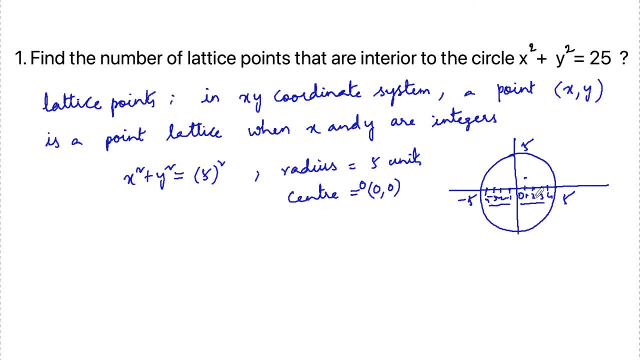 So total, there are inside 4 plus 4, 8,, 9 points are there. Among the 9 points we need to select one point and then again on y-axis, also, in total there will be 9 points And again we need to select one point so that the total number of ordered pairs from this. 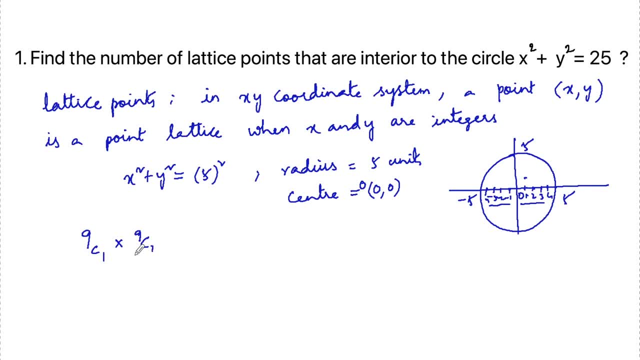 total four points, and four points on the x-axis and y-axis are 9c1 and 9c1.. we can observe that there are some points which will be outside and on the circle. So, if I can draw these lines, we can observe that the points which are